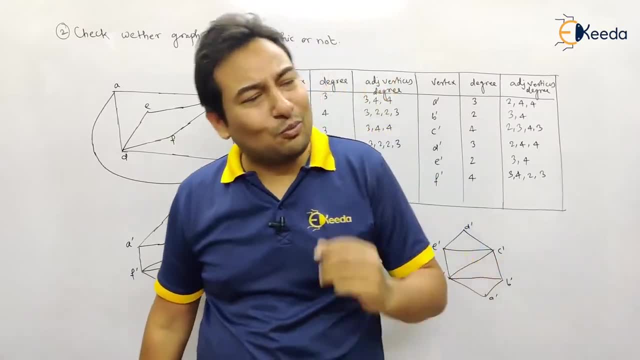 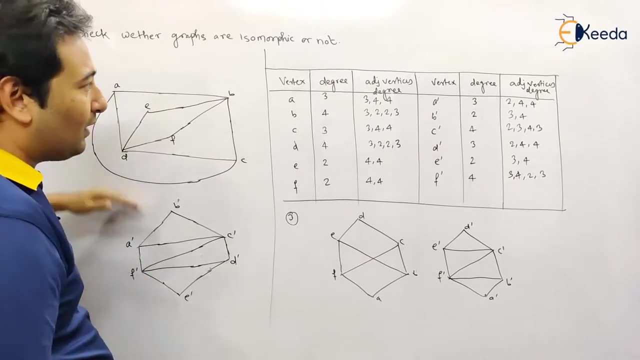 Is it how it is possible? three conditions satisfied, still it is not isomorphic. To prove my point, the example is in front of us. This is the next problem. we are going to check whether it is isomorphic or not. First of all, let us count number of vertices. 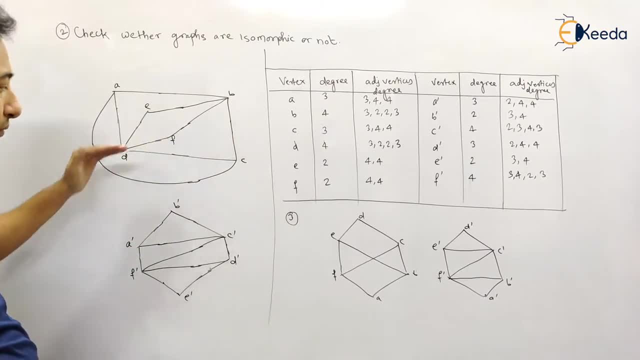 If you check, the number of vertices are 6 in both the graphs. Next, Number of edges. let us count the number of edges: 1, 2,, 3,, 4,, 5,, 6,, 7,, 8, 9.. 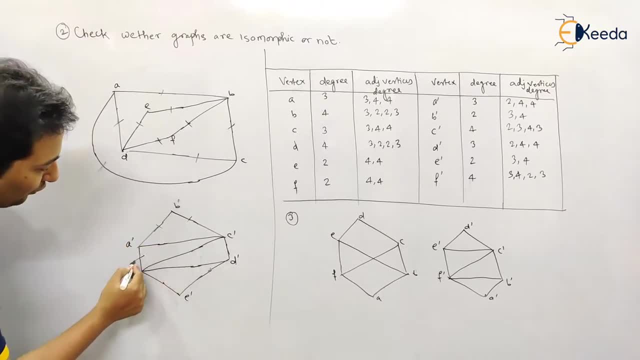 So in the first graph, 9 edges 1,, 2,, 3,, 4,, 5,, 6,, 7,, 8, 9.. Again, the number of vertices are same, number of edges are same. 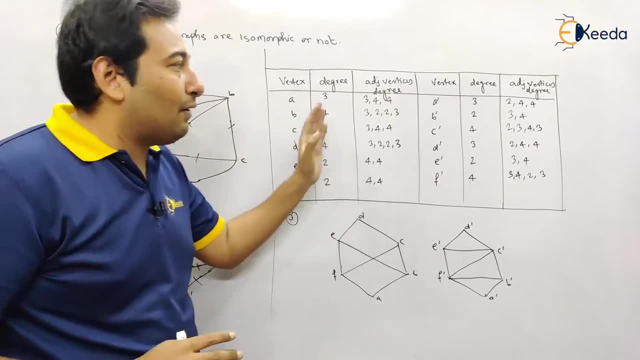 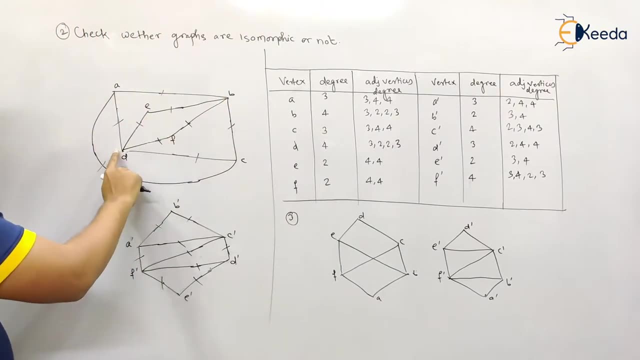 Let us check For simplification. I have already created this table just to save the time in the video. A has degree 3, B has degree 3, it has degree 2,, 2,, 4, 3.. Likewise, this is 2,, this is 2, 4, 4,, 2, 4 and 3, so this is listed down here. 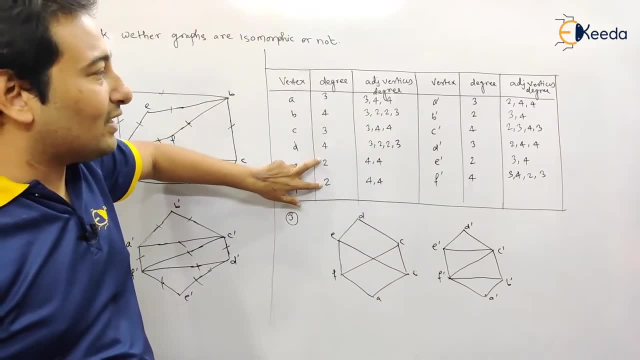 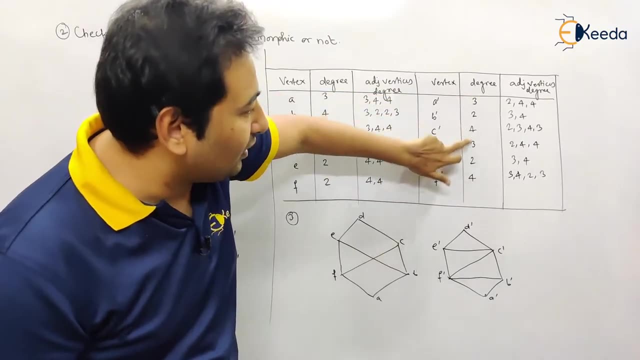 Now let us check how many vertices with degree 2.. So here there are 2 vertices with degree 2, here also 2 vertices with degree 2, 2 vertices with degree 3, 2 vertices with degree 3, 2 vertices with degree 4, 2 vertices with degree. 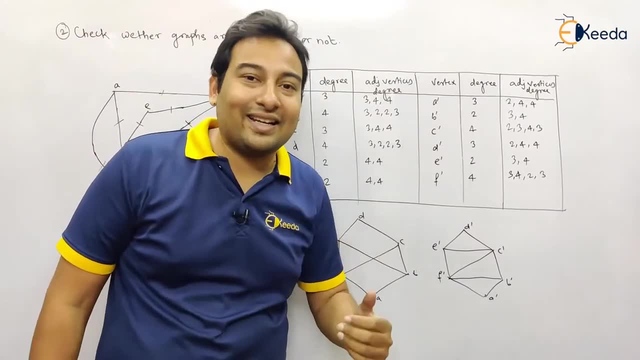 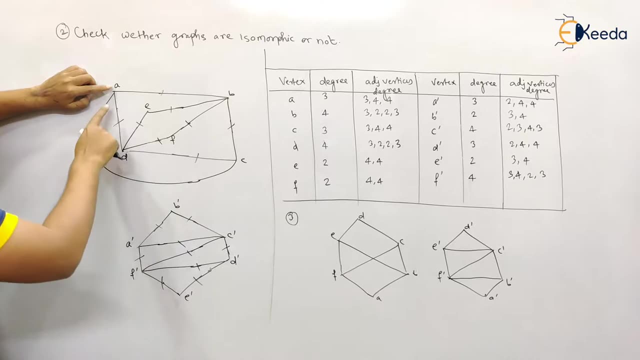 4.. That means condition number 3 is also satisfied. Now let us check the last criteria, that is adjacency. Now for mapping A. A has degree 3 and A adjacent degree are. its adjacent are this: that is, its degree is 4, its degree is 4 and its degree is 3.. 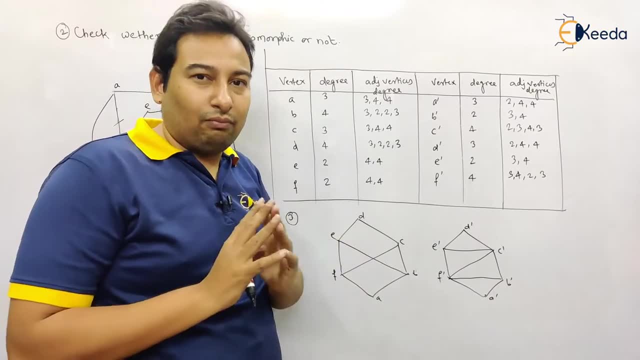 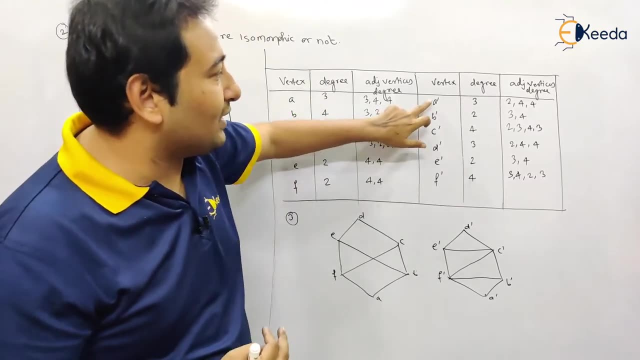 That means 3, 4, 4.. I hope you know how to make this table right Now: 3,, 4, 4.. Now I want to map A. For mapping A, I have two options. Either I can go with A dash and D dash. 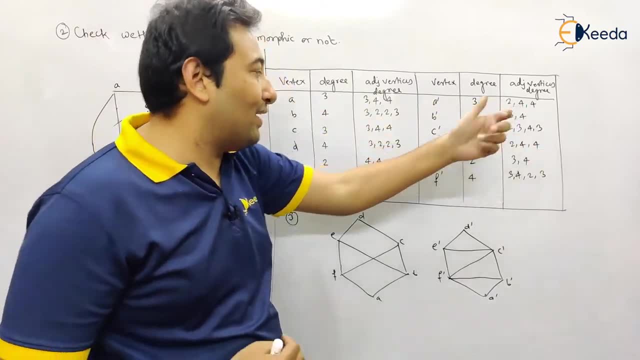 Now, if I will check its adjacent degree, it is 2, 4, 4,, 2, 4, 4.. Let us check A dash and D dash. See here A dash: the adjacent is 2, here it is 4 and here it is 4.. 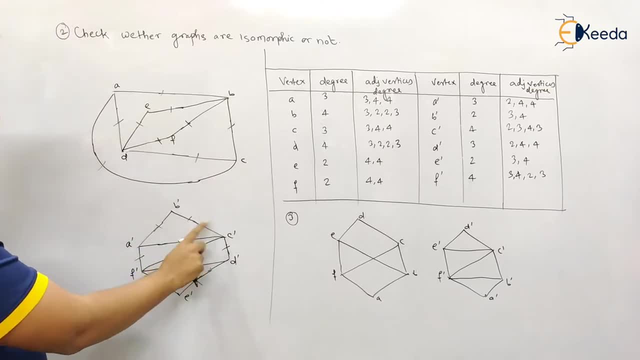 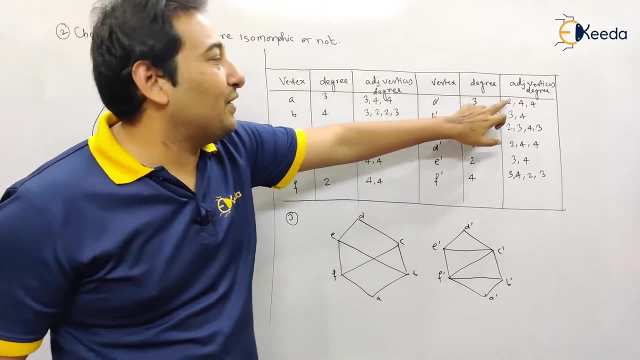 So 2,, 4,, 4.. And the next option is D dash: Here it is 4,, here it is 4 and here it is 2.. That means, here we are getting 2,, 4, 4,, 2,, 4,, 4, and here we are getting 3,, 4, 4..